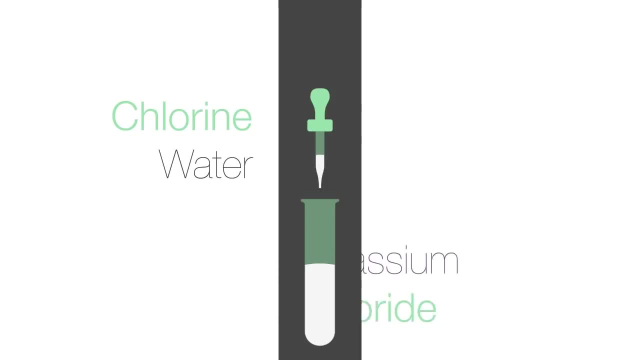 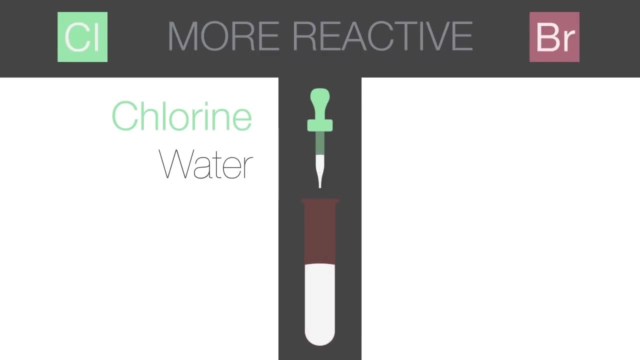 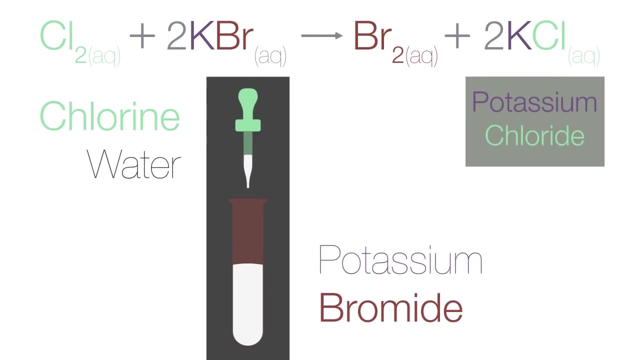 When we add chlorine water to an aqueous solution of potassium chloride, no reaction happens, Since chlorine is more reactive than bromine. chlorine will displace bromine in potassium bromide, producing potassium chloride and liberating bromine. The resulting solution is a solution of potassium chloride and potassium iodide. The solution: 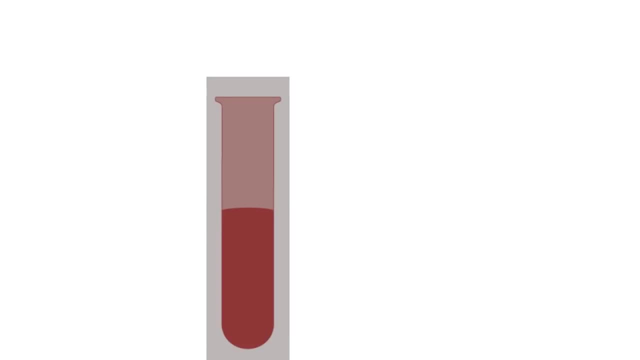 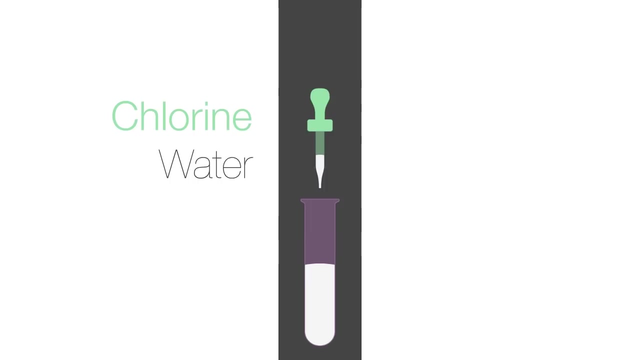 is a solution of potassium iodide and potassium iodide. The solution of potassium iodide is reddish brown due to the presence of bromine. A similar observation occurs when chlorine water is added to an aqueous solution of potassium iodide, Since chlorine is more reactive than 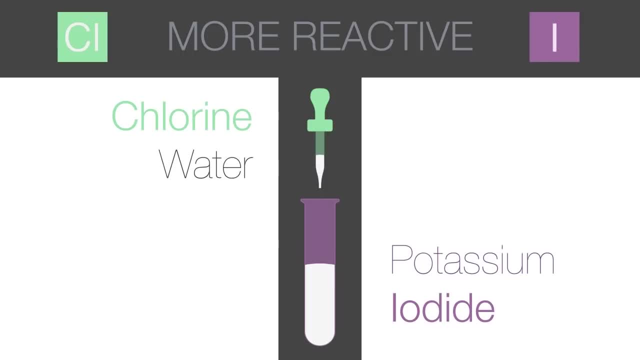 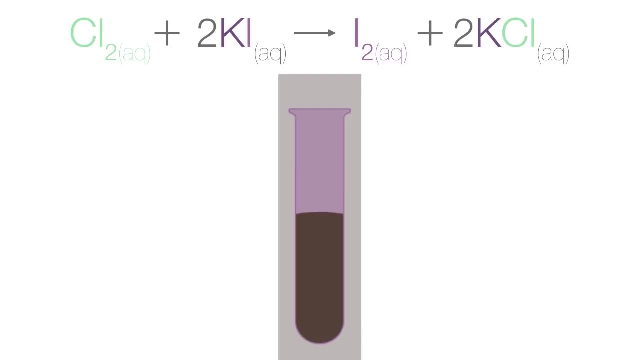 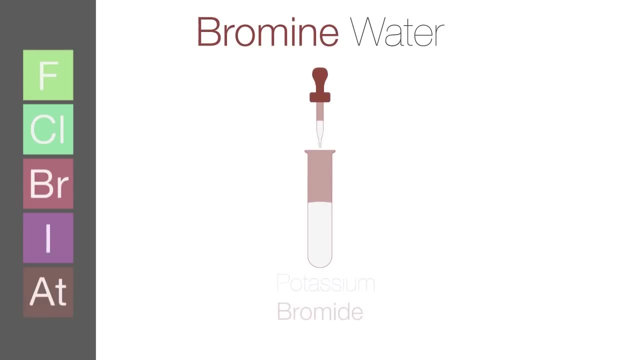 iodine, a displacement reaction will occur to liberate iodine. according to the reaction below, A dark brown solution is produced due to the presence of iodine. We can see How Bromine Works when bromine water is added to the same three aqueous solutions. 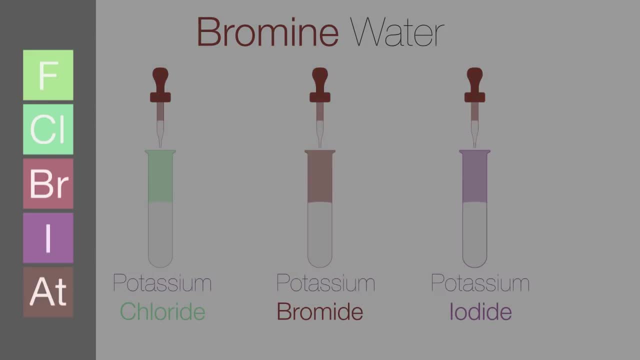 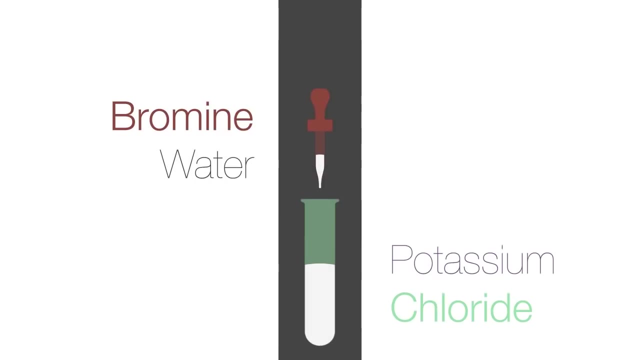 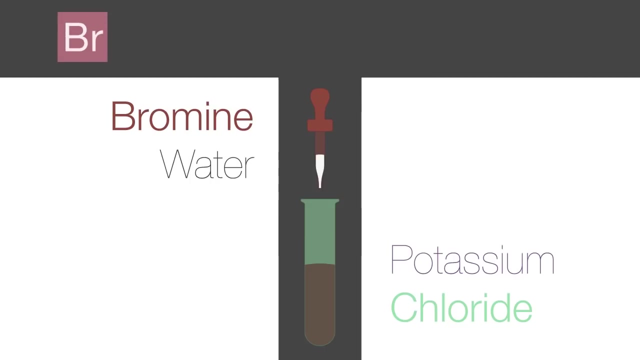 Please pause the lesson to think about this and resume once you are done. When we add bromine water to aqueous potassium chloride, this causes the solution to turn reddish-brown, but no displacement reaction occurs, as bromine is less reactive than chlorine. 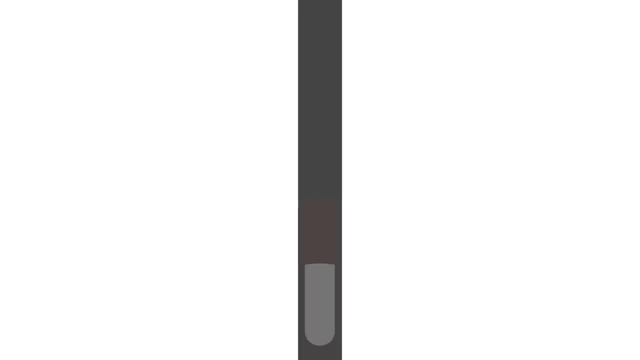 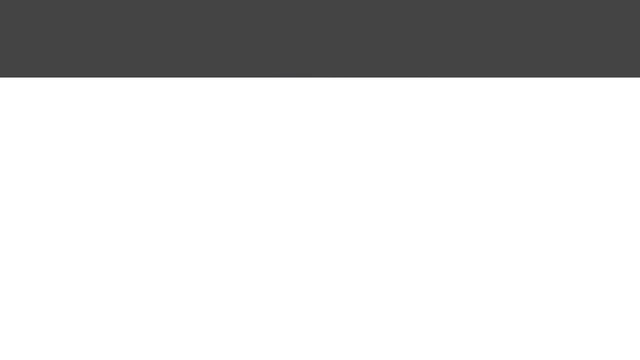 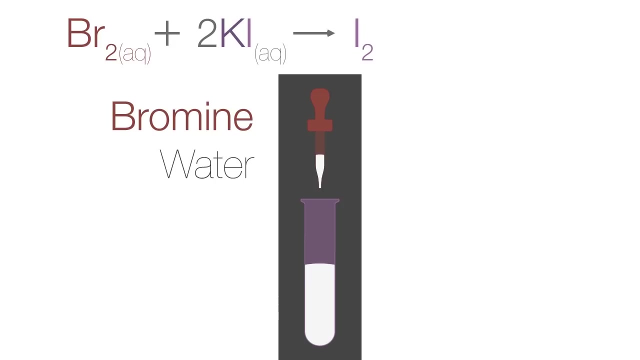 No reaction occurs when bromine water is added to aqueous potassium bromide. As bromine is more reactive than iodine, it will displace and liberate iodine in potassium iodide. Therefore, a dark-brown solution is produced due to the presence of iodine. 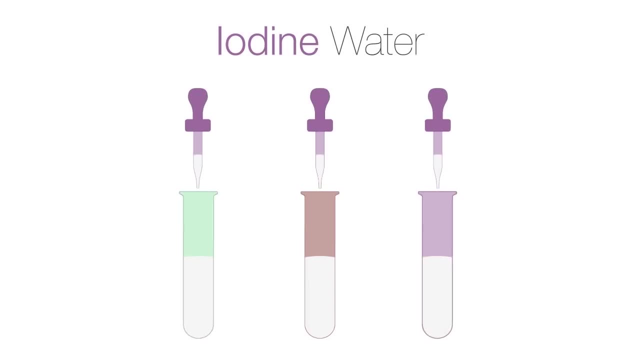 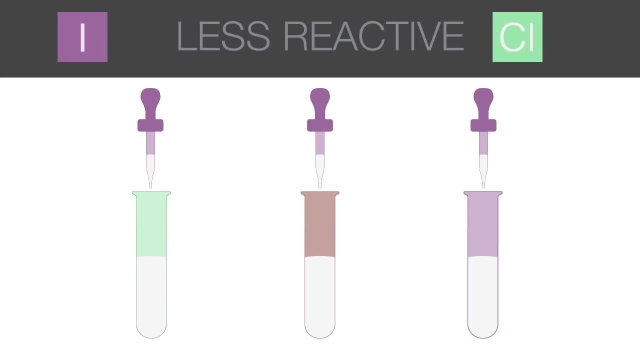 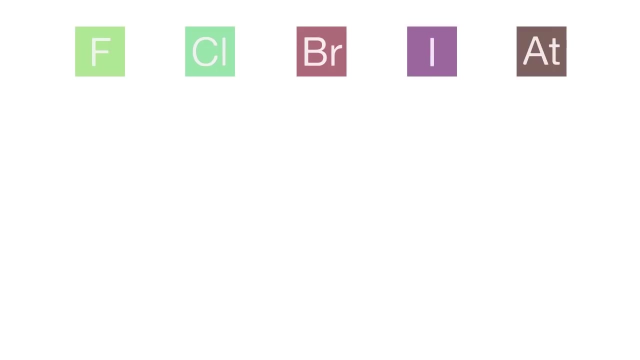 If we added iodine to the same three aqueous solutions, no displacement reactions occur, as iodine is less reactive than both chlorine and bromine. Halogens can react with certain metals to form metal halides. A very common metal halide is sodium chloride or regular table salt. 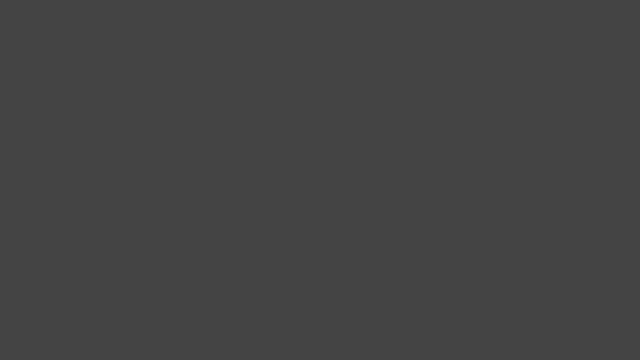 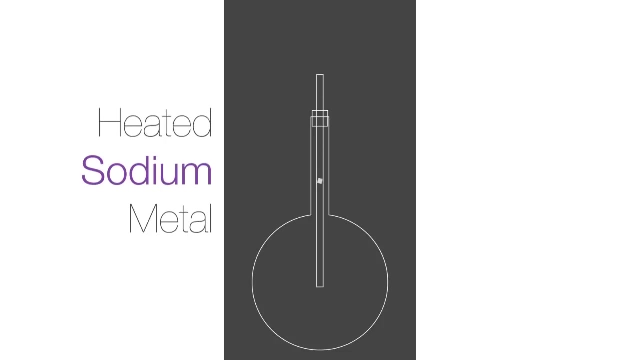 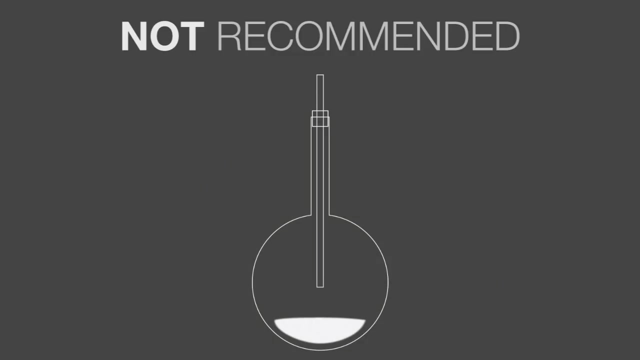 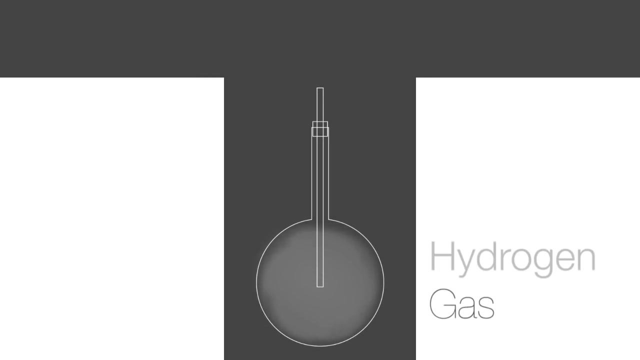 Sodium chloride is extracted from the sea or from salt mines. Sodium chloride can be produced from the reaction of heated sodium metal with chlorine gas. Since it is a highly exothermic reaction, it is not recommended that this be done in a laboratory. Halogens can react with hydrogen gas to produce the corresponding hydrogen halide.